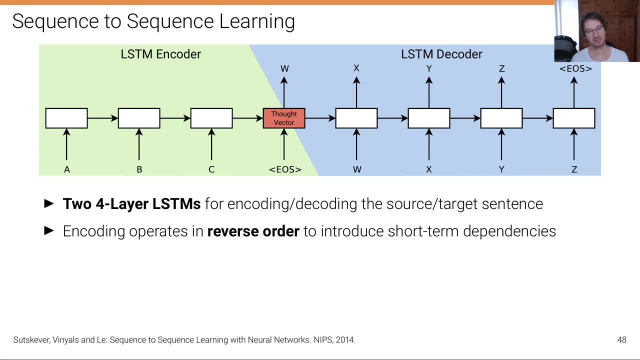 Then we reverse the order of the input sentence And this is advantageous because it introduces short-term dependencies, because we end with the first word and then the decoder starts to decode with the first word in the target language. And by reversing the input sentence you get shorter dependencies because the first word in the input sentence is likely related. 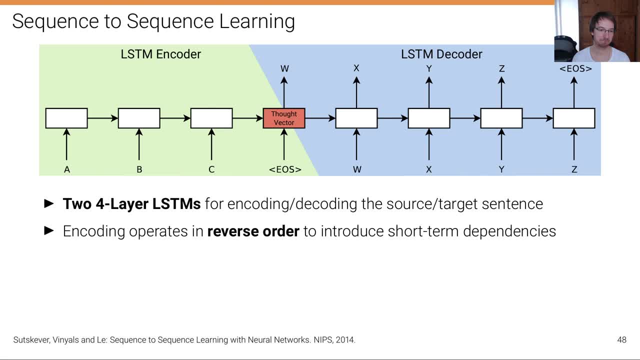 to earlier words in the output sentence, But otherwise is a simple LSTM. So here's an LSTM that processes this reverse ordered words word by word. So the words are embedded in a word, a distributed word representation, and there's a hidden state that is carried forward through this recurrent neural network. 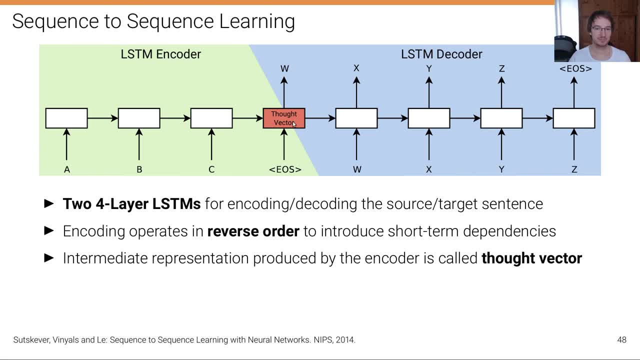 And then there's an intermediate representation that's called a ford vector. This is the representation that stores the meaning of that sentence. that shall be translated. So once we reach the end of symbol, end of sentence, symbol we produce, we have the ford vector. 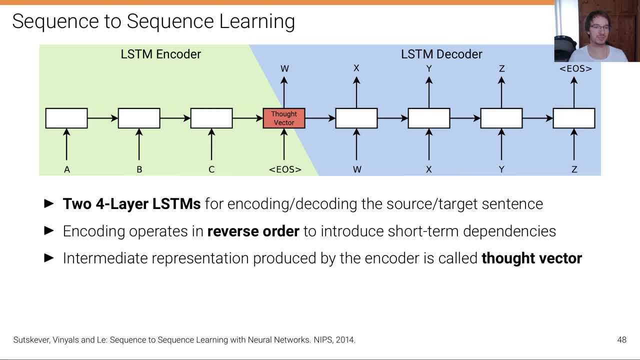 as the hidden representation. It's a global representation of the input sentence And then that ford vector is decoded. And the reason why we have this interface of the ford vector is that the input sentence and the output sentence may have a different length And also the word order is very different in different 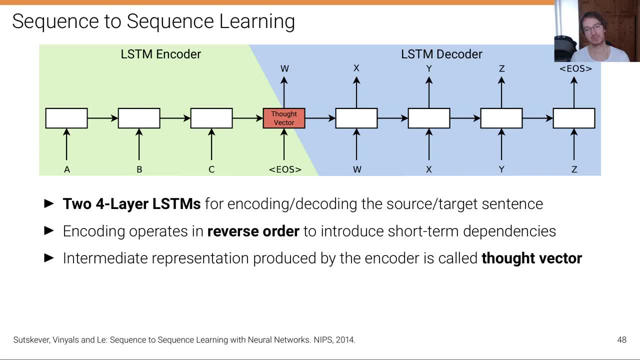 languages, depending on the grammar of these languages. So we create a global representation of the input sentence, the ford vector that is passed to decoder. And it has long been believed in a community that such a simple system cannot work because it's impossible. People have claimed it's impossible to generate a ford vector, a global representation of. 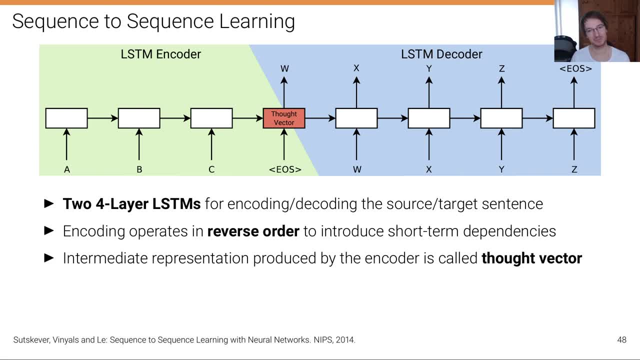 a sentence that captures enough to decode it well in the target language. But then this was the first paper that demonstrated that this is possible, surpassing all of the existing techniques that have been developed so far. So they used a wording embedding of 1000 dimensions and the decoding was done via BeamSourcecom. 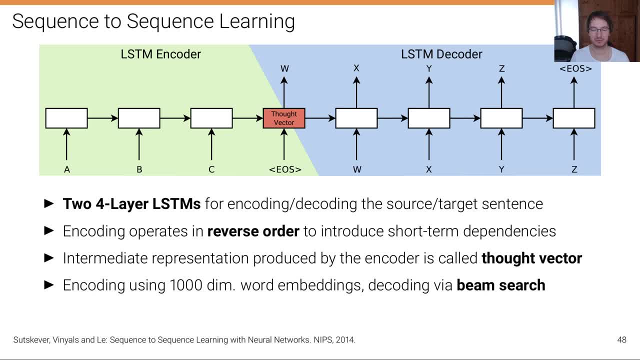 Thank you, search, which we're going to have a short look at in a minute. It was the first end-to-end system that outperformed all of the state-of-the-art models and was also the first system that demonstrated that this is really possible at large scale and that led to deployment. 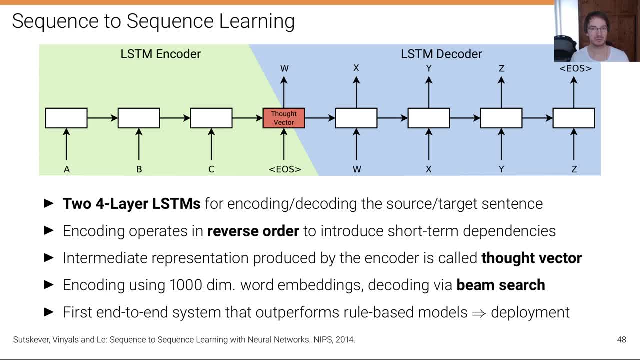 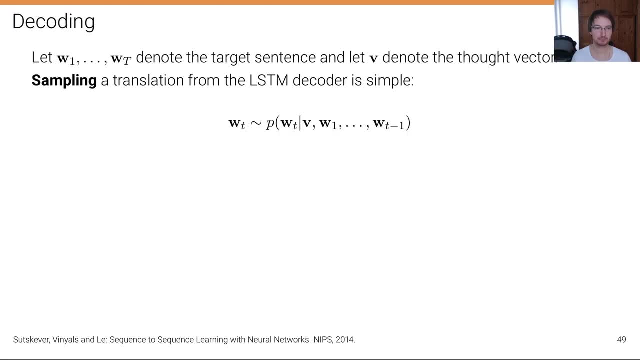 So that was the time then, in 2015, when, for instance, Google completely transitioned to neural from the traditional language translation models. they had to neural machine translation models in 2015.. So let's talk about decoding. How can we do decoding? Well, let w1 to wt denote the target. 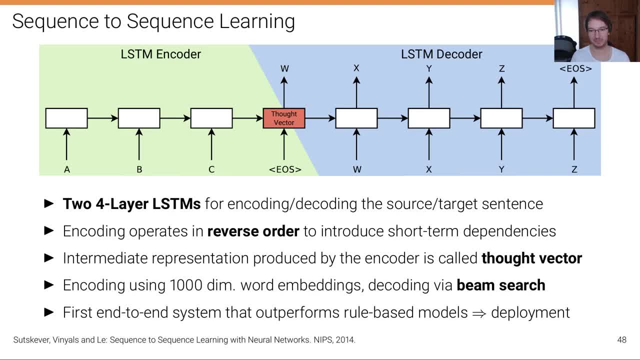 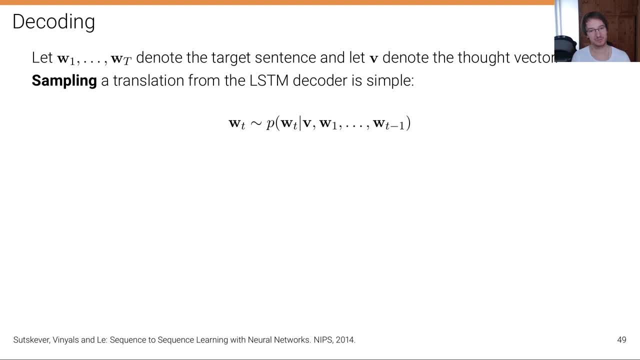 sentence and let v denote this fault vector that we have here in red, Then sampling a translation from the LSTM decoder is really simple, because we have this autoregressive nature that we can just sample a new word from the distribution that is predicted by the LSTM, given the fault vector and the previous words. 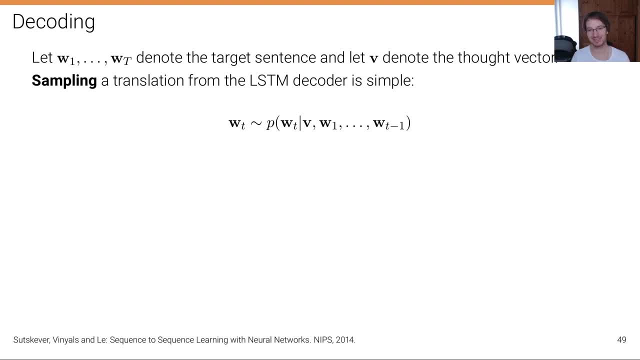 where the previous words are summarized in this hidden state in the case of an LSTM. But this is not what we want to do in translation. What we want to do is we want to compute the most probable translation for an input center, For example. we want to find the most probable translation for an input center. 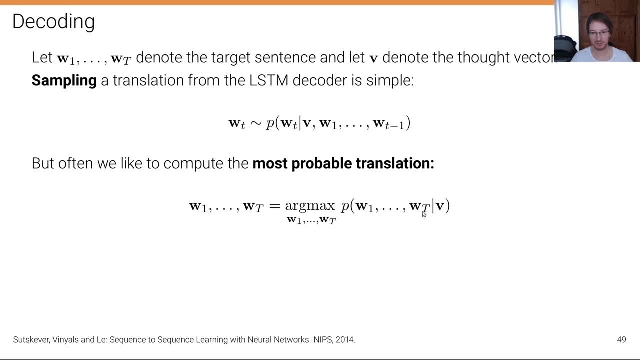 So in this case we want to find the most probable translation for a sentence, or in other words, we want to find w1 to wt that maximizes p of w1 to wt, given the fault vector v. Now this is very costly because there's a large number of possibilities for possible translations. 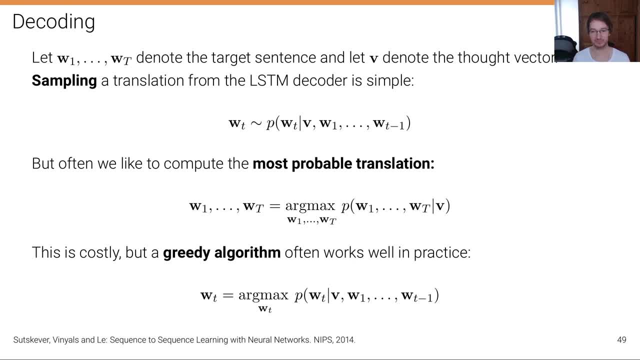 So searching that exhaustively is intractable. algorithm might actually work well and it often does in practice. and a greedy algorithm is one which basically word by word, finds the best word that maximizes the probability up to that word. so we take argmax over only wt if we compute the next word, t, given v, and all the previous words. 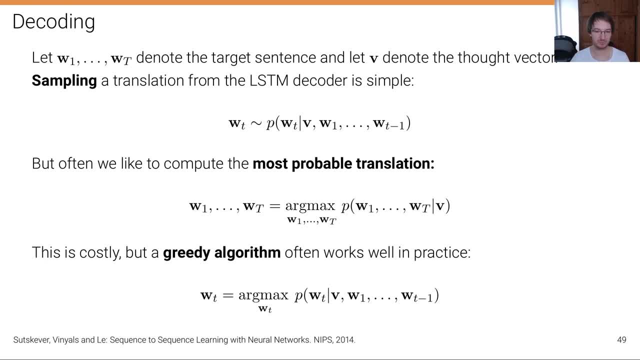 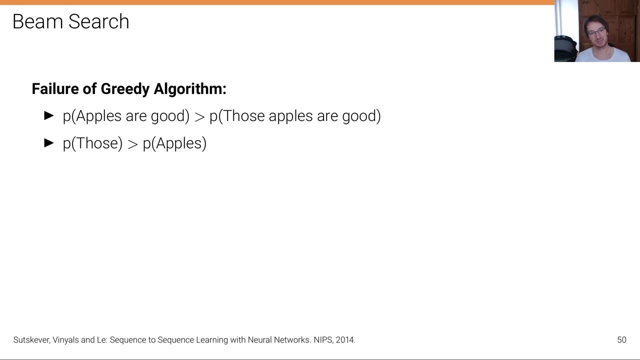 before the word t, so this is called a greedy algorithm. it's important to note that these two are not the same. they don't lead to the same result, but the greedy algorithm is often a good approximation. so here's an example of a failure case of a greedy algorithm. let's consider the 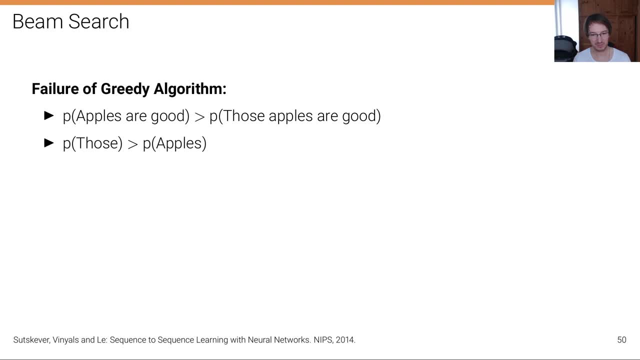 sentence apples are good and the sentence those apples are good, those apples are good. the probability of apples are good in a training corpora might be larger than the probability of those apples are good, because apples are good occurs more frequently. however, there is more sentences in the training corpora that start with those compared to apples. 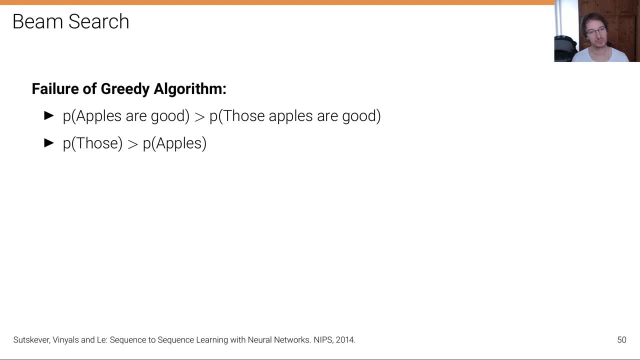 so the probability of the sentence those like the partial sentence those- is bigger than the probability of the partial sentence apples- the sentences that start with apples. so if we do greedy decoding then we would start with those, even for the probability of apples is the probability of apples are good and the probability of apples are good is greater than the probability of apples. 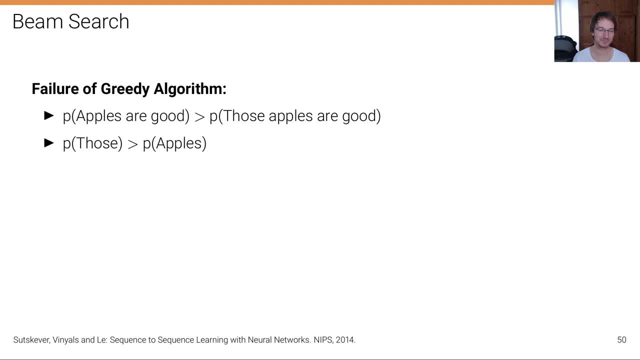 are good is bigger than the probability of those apples are good, And this is where beam search comes in. Beam search is somewhere in between. It's better than a purely greedy algorithm, but it's still only an approximation to the true solution that searches over the entire search. 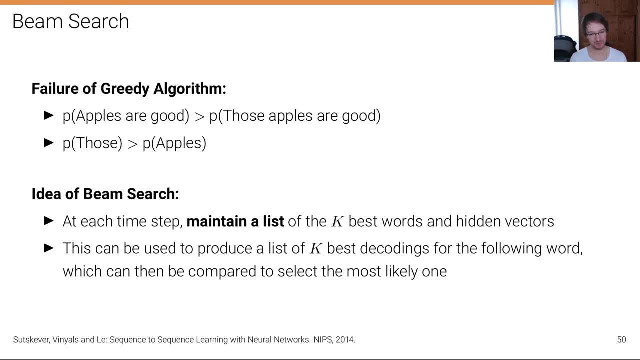 space And the idea of beam search- and that's also what is done in this paper for decoding- is that at each time step we maintain a list of the k best words where k is a hyperparameter of beam search, And we keep a list of these k best words. 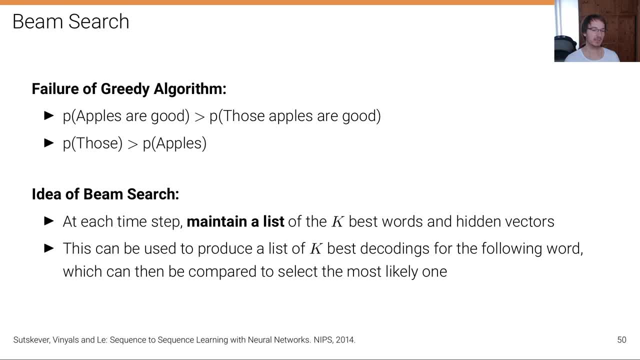 and the best of the corresponding hidden vectors, And this can be used then to produce a list of k best decodings for the following word. So for all of these k best words with the hidden vectors, we can look at all possible next words and multiply the probabilities and then 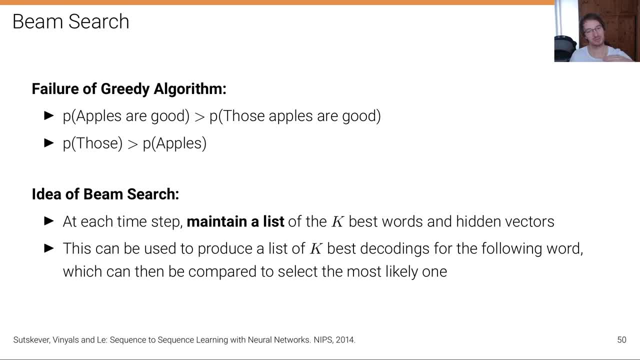 find the best combination And then just get a sorted list of these best combinations and shorten that list again to k for the next step, and so forth. And so this is why it's called beam search. We always keep a beam of k solutions. 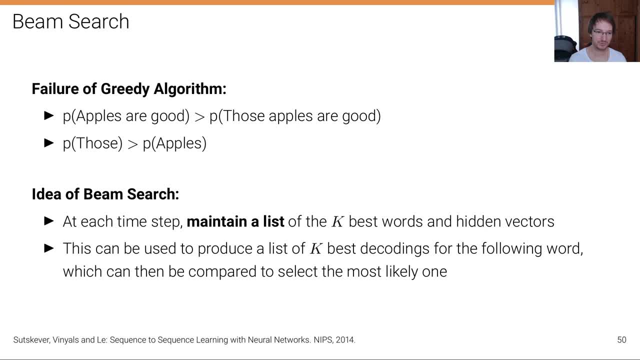 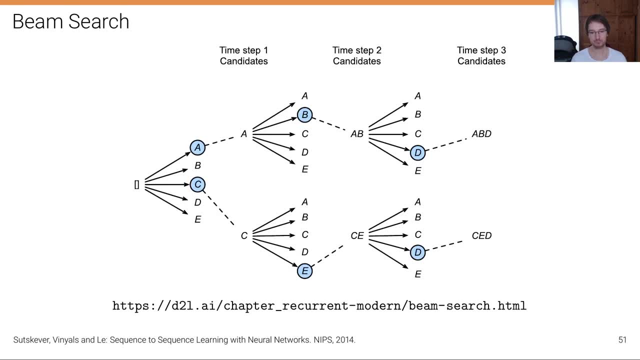 And through that we can come up with better solutions compared to naive greedy search where we're still just doing an approximation and it's still tractable. Here's an illustration. There's also the website where you can find a little bit more. 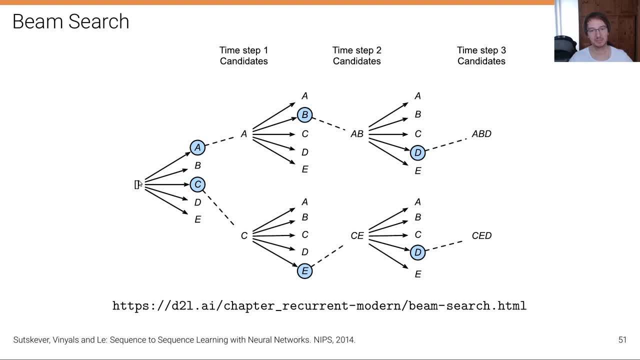 explanation, but it's very simple. We start here with an empty sequence and then we have a, b, c, d, e as candidates And a and c are most likely. So with a beam of size 2, we keep track of a and c. 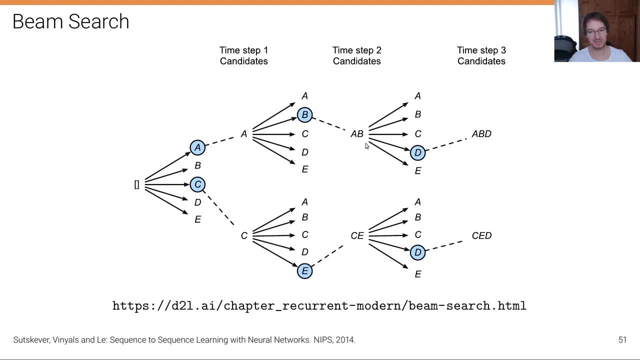 And then for a: b is most likely and for c: e is most likely. And then we continue: a b and c e. So we maintain always this short list of two hypotheses, And it could of course also be the case that here a b 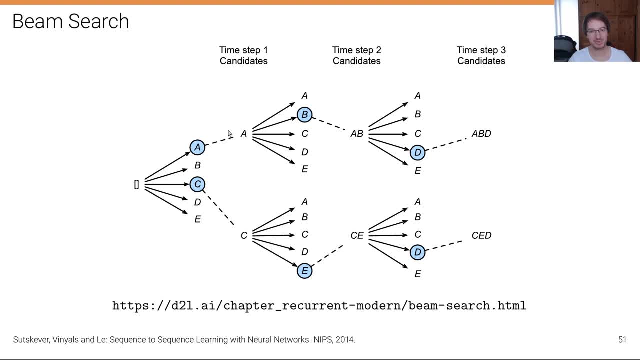 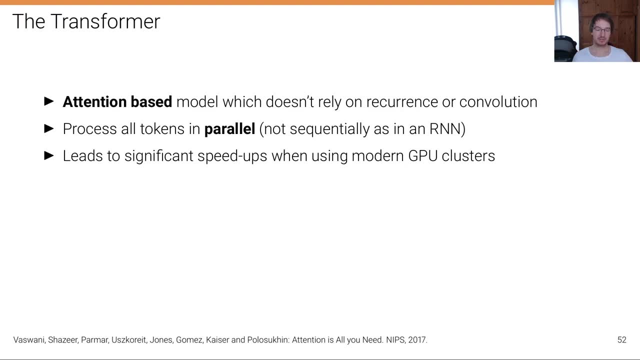 and a c are both more likely than c? e, in which case we would continue with a, b and a c here. Now, this was a big step. The paper that I mentioned before made a big step, and it led. 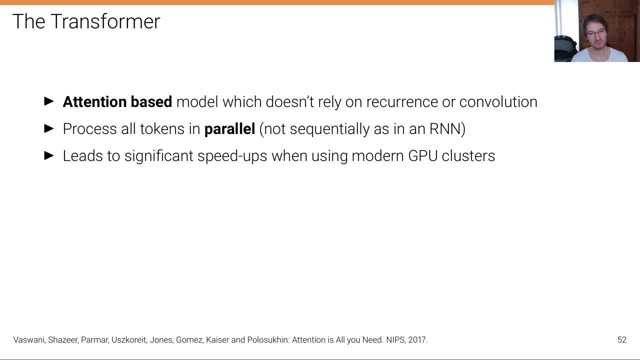 The industry to change the algorithms that we were using in practice. So it meant really that it started working. Neural machine translation started to have an impact in practice. But then, in 2017, there was another big step and it was the transformer paper that completely changed. 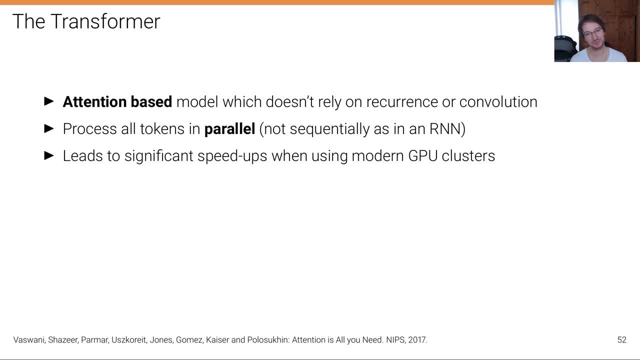 the architecture of previous neural machine translation models into a purely attention-based architecture. So the transformer is an attention-based model and we'll come to that- which doesn't rely on recurrency or convolutions. There's no RNN or no convolutional layers. 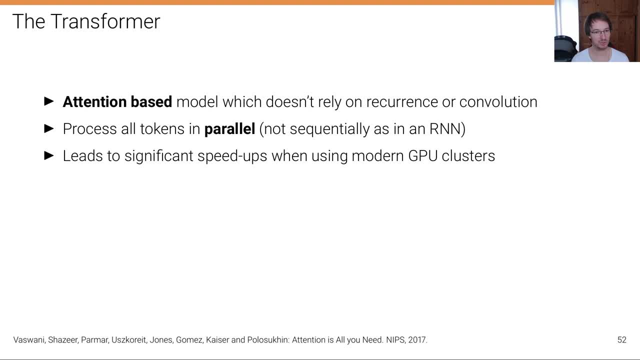 in the model I'm going to show you. It's just an attention-based model, And the advantage of an attention-based model, over a RNN, for instance, is that there is no sequential dependencies. You don't need to wait for the previous words to be computed. 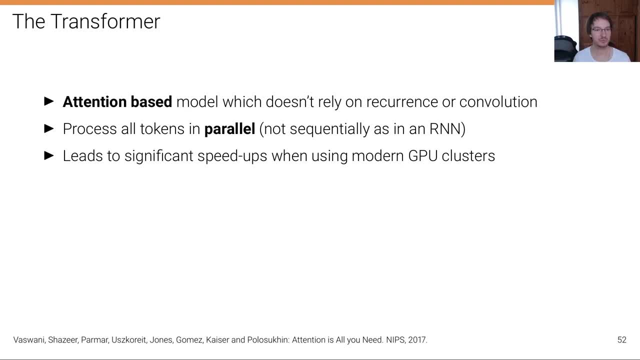 until you can compute. You can compute probability for the current word, But all the tokens can be processed in Perl, And it's advantageous because nowadays all the computational gains are through Perlism, And so we want to have our models also as Perlizable as possible in order 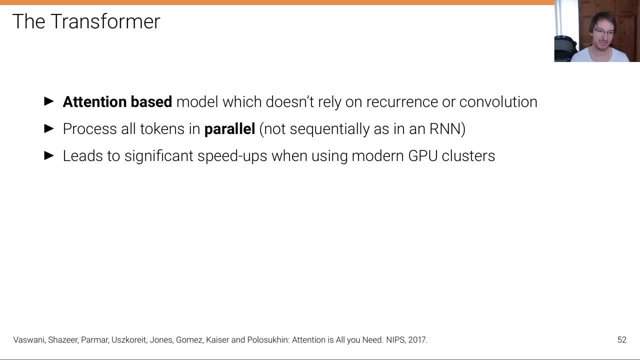 to take advantage of the massively Perl hardware that's available today, So that leads to significant speedups when using modern GPU clusters, And that's what this paper exploited. This is also a paper from Google. Self-attention is what has been used in the transformer. 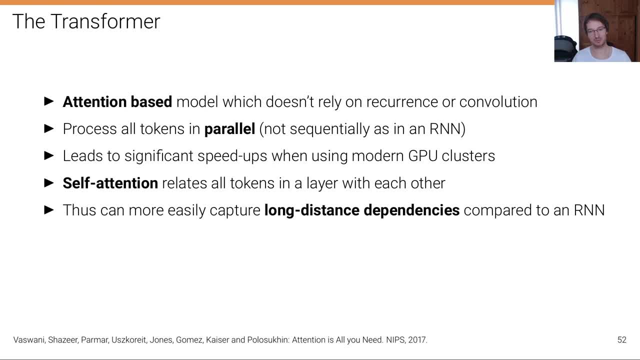 And self-attention relates all the tokens, all the words in a layer with each other, which means not only that this can be computed in Perl, but it also means that it can more easily capture long distance dependencies, compared to an RNN, where 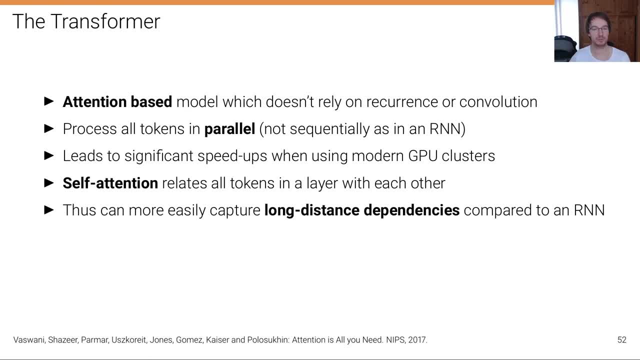 these long distance dependencies have to be carried over the time steps, through the hidden state with all these problems of managing gradients. Here we're doing Perl processing And therefore we can directly relate any element to each other in the sentence, And transformer-like architectures have now replaced. 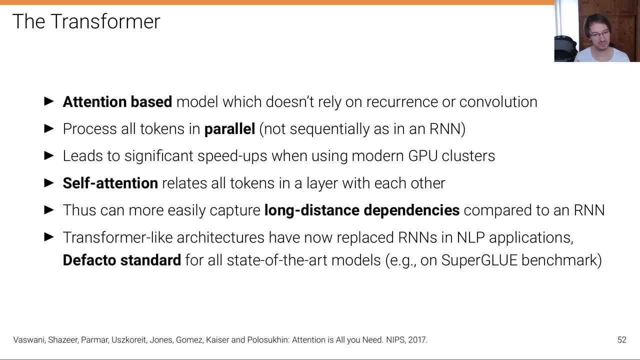 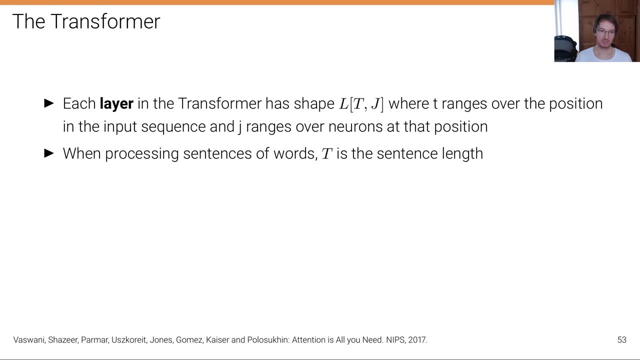 RNNs in NLP applications almost entirely, Thank you. They are de facto standard for all state-of-the-art models, for instance on the superglue benchmark, which is one of these standard benchmarks to evaluate machine translation performance. So let's have a bit more closer look. 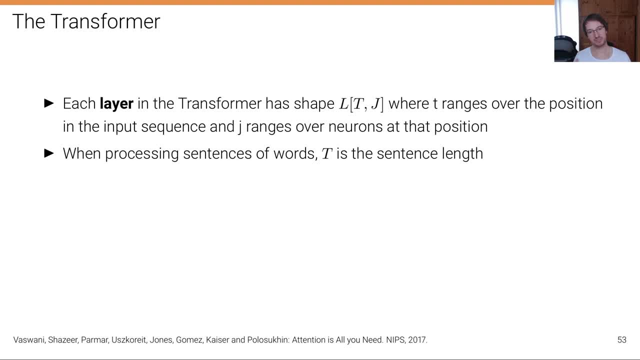 into what the transformer does. Each layer in a transformer has a shape of L, where we use L for layer. This is Einstein notation. now that I'm using L, of t, of t and j, where t ranges over the position in the input sequence and j ranges over the. 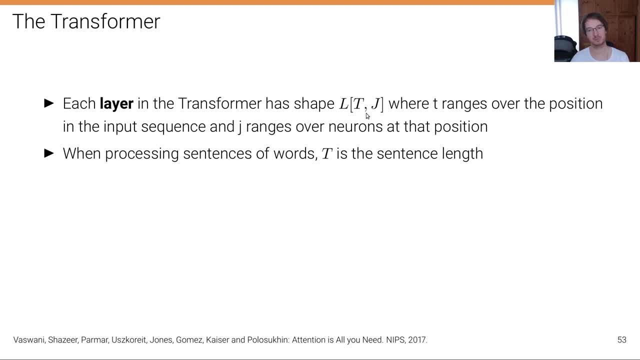 neurons at that position. This is basically a matrix where, for each position, for each word, we have a vector, a word embedding, And when processing sentences of words, t is the sequence length. So this is basically the same shape as in an RNN: It's a sequence. 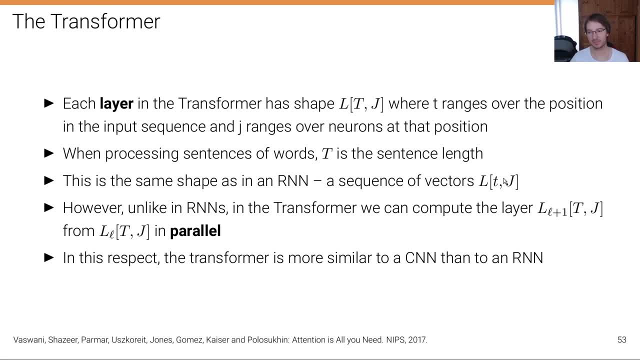 of vectors. So here we have a sequence of vectors: Little t, big J is a vector. However, unlike in RNNs, in the transformer we can compute the layer, the next layer- L plus 1, from the previous layer, completely in parallel. That's what I mentioned before. So we go from: 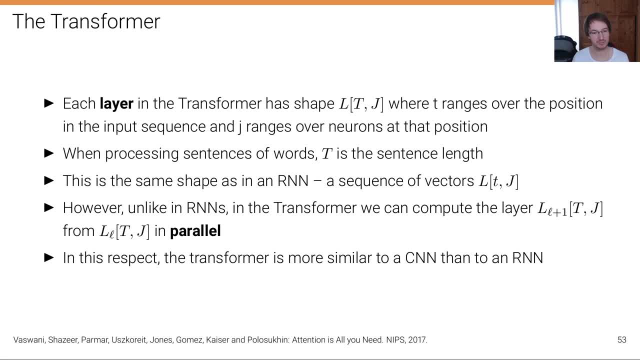 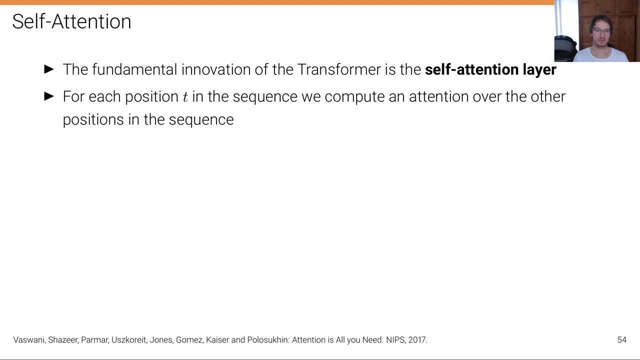 one tensor to the next tensor completely in parallel, without the sequential. So in this respect the transformer is actually more similar to a CNN than to an RNN, but it's different from a CNN because it has attention and it doesn't do convolutions. The fundamental 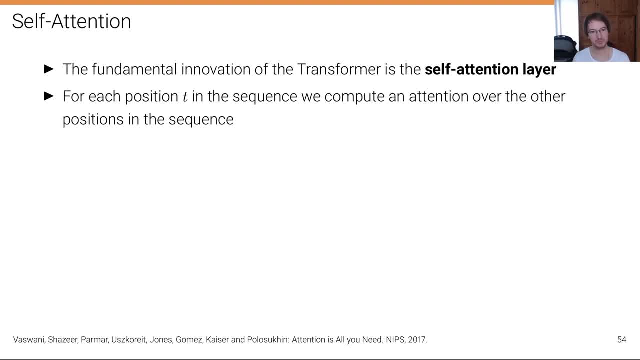 innovation of the transformer is the self-attention layer. For each position t in the sequence, we compute an attention over the other positions in the sequence. We'll make this more formal on the next slide. And then the transformer uses multiple heads. So initially we tried to have a single head, but then they split up the computation. 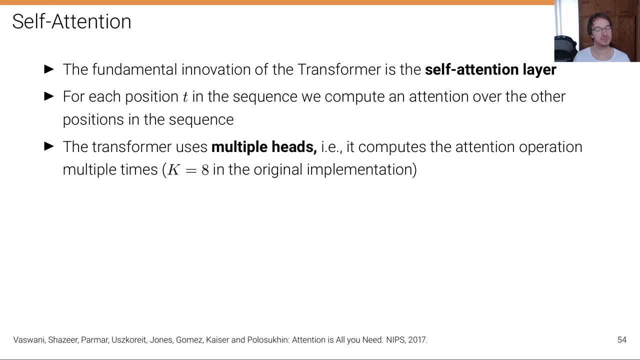 into multiple heads because this gave them empirical benefits. So there's eight different heads in the original implementation, each of which computes its own attention operation. It's not very well described in the paper why they use multiple heads, but it just empirically works better. 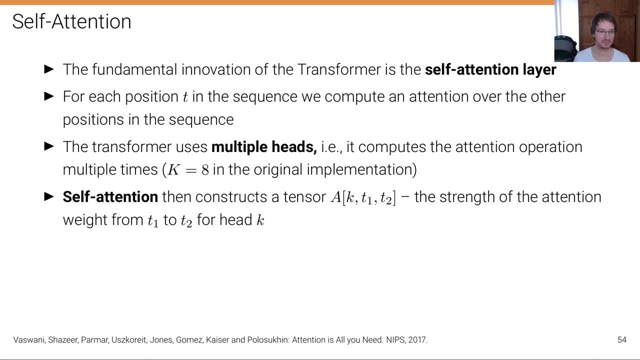 And then the self-attention is constructed, constructs a tensor, we call it a for attention, with indices k, t1, and t2, which specifies, for head k, in this case the head index from 1 to 8, the strength of the attention weight from t1 to t2.. 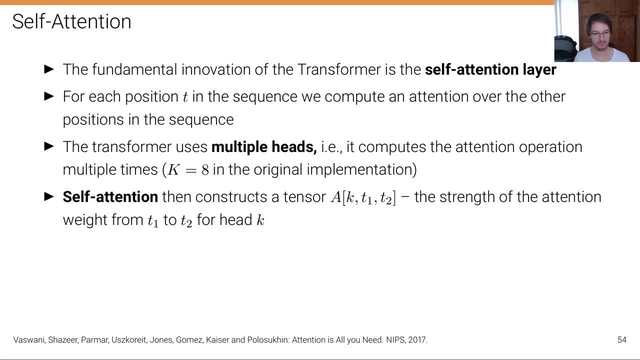 So the attention that t1 pays to t2, that word t1 pays to t2 in a particular layer of the transformer for a particular head k. so that's very abstract but we'll make it more formal and in the paper they used an embedding dimension for each word as a word. embedding dimension of 512. 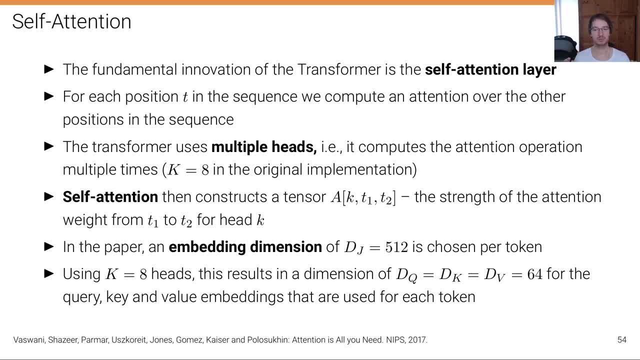 token means word. this is a word model, so, per token, 512 dimension, and they use eight heads. so, um, that they use, then? because we have eight heads? they used for the query and the keys and the values that this attention, self-attention- layer utilizes. they use 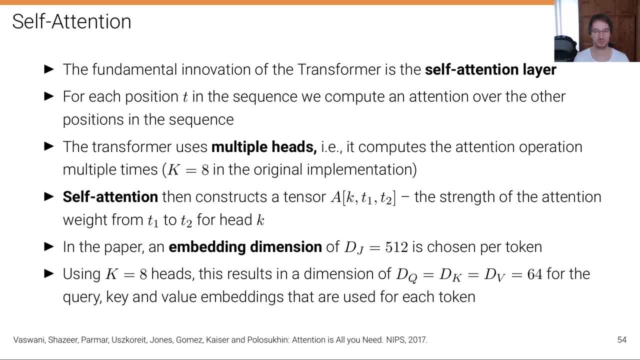 64 dimensions. 64 times 8 is 512. so we break the problem from 512. they do computations at 64 dimensions, but they do it eight times and then they concatenate again to get 512.. in fact they concatenate and they do a fully connected layer. so they could use a different. 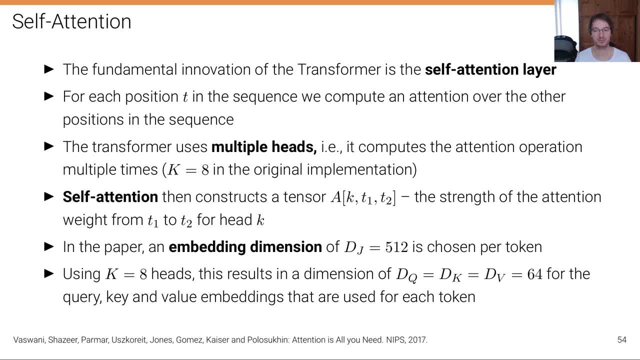 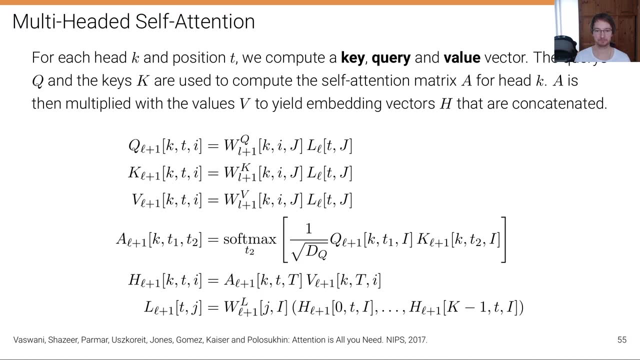 intermediate dimension, but they wanted to keep it comparable, so they used exactly 512 divided by 8.. and this query, key and value embeddings are properties of this or values of the self-attention layer that we're going to talk about. so this is the transformer on one slide in terms of equations. 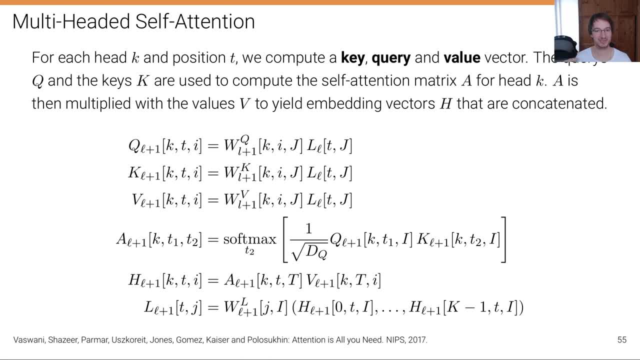 so the transform itself is a self attention layer, and it's not exactly correct. it's a self-attention layer. the transformer has multiple layers, but one of these layers, the most complex one, is the self-attention layer, the multi-headed self-attention layer, and this is what is on this slide. 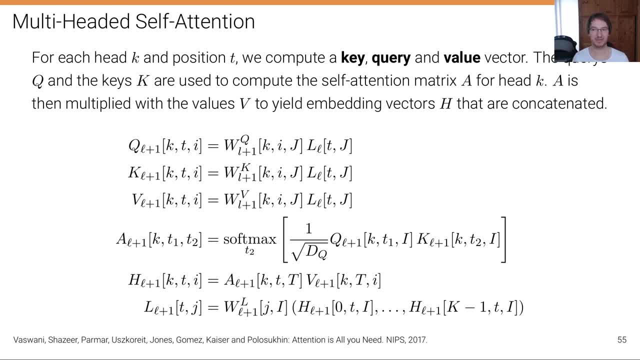 so for each head k and each position, for each word in a sequence, we compute a key query and value vector. these are the 64-dimensional vectors Q, the keys we call K, and these are used to compute the self-attention matrix A for that hat. 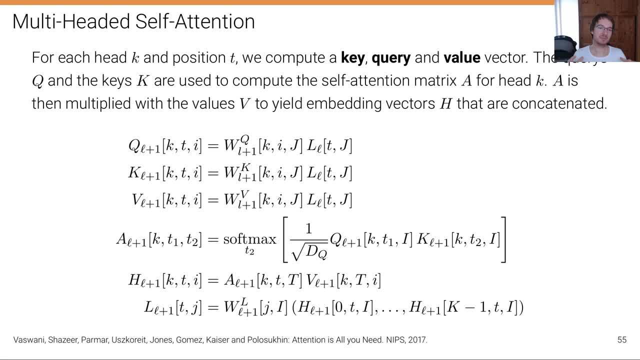 And then A. this attention matrix is multiplied with the values B to yield embedding vectors H that are then concatenated. These are the 64 times 8.. They concatenate eight of them and they are then multiplied with a matrix to yield the output of that layer. 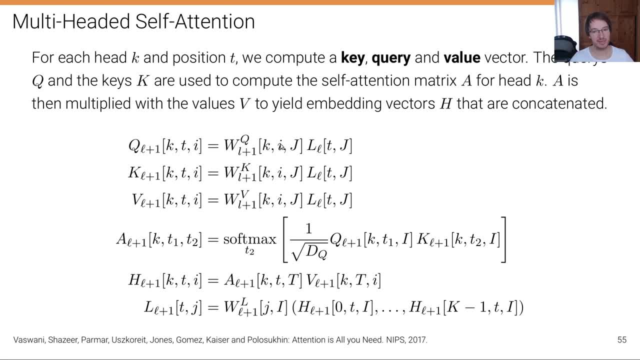 And so this is what it looks like in Einstein notation. So we start at the bottom, where we have just words represented maybe as one-hot vectors or word embeddings of one-hot vectors. So we have some word embeddings of these one-hot vectors and we multiply these. so this is at time. 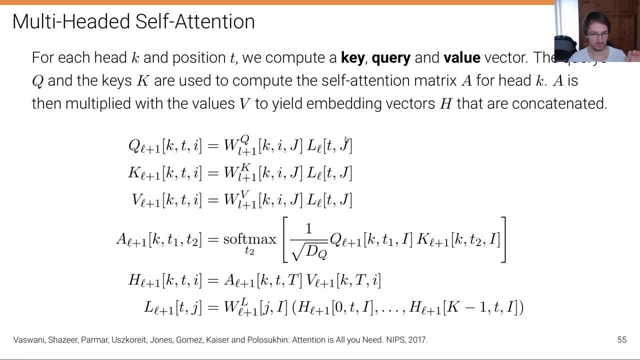 step t, we have a vector. this j is all of the elements of that vector, and we multiply this, add layer at the first layer with a matrix, W, WQ, to get a query vector. So this runs over i. So I could have used capital. I's here as well. 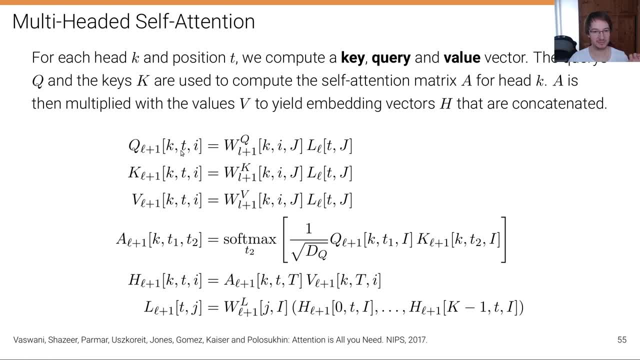 We have this query vector, we have, for hat K at time, step t and that runs over i and this is 64 dimensional. So we go from 512 dimensional j to 64 dimensional i using this matrix multiplication And we have different matrices, three different matrices: one for the so-called query, one for 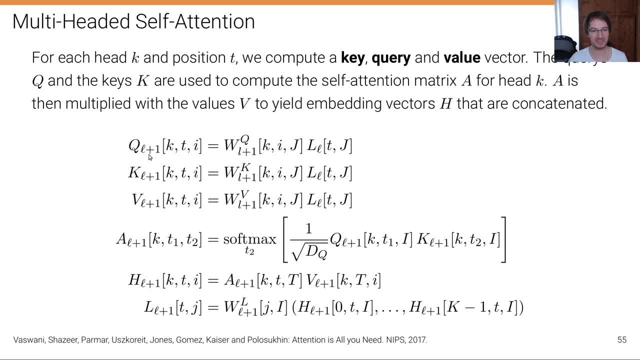 the key and one for the matrix. So we have three different matrices: one for the so-called query, one for the key and one for the matrix. So we get query, key and value vectors of 64 dimensions for each hat and for each word. 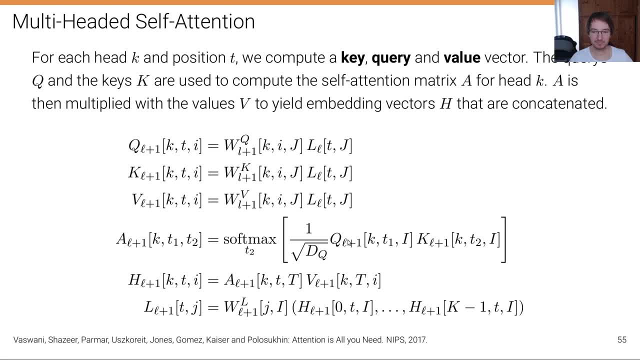 And then we multiply the query and the key. If they are similar, then this leads to a strong activation of the attention matrix A. There's some normalization factor here as well, And then we do a softmax over T2.. So this is basically here. you can see this goes over T1 for Q and T2 for K. 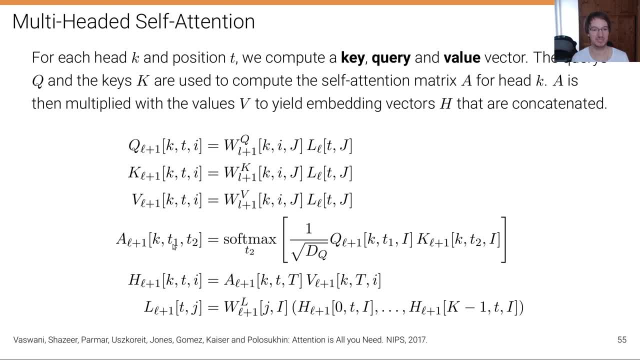 And so we get this matrix of T1 attends to T2 relationships here for hat K And it's over all the. this is a vector multiplication, it's over all the elements of these query and key vectors And then the softmax to normalize. 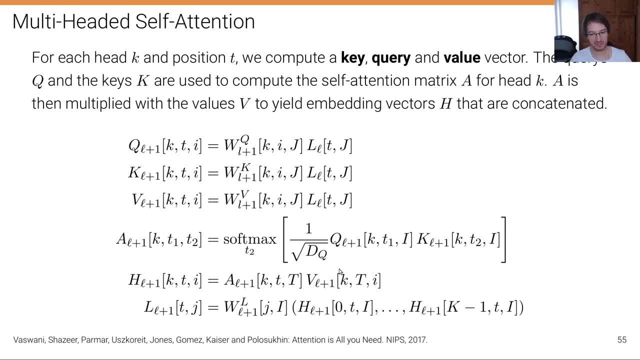 And so then we have this attention matrix and we multiply this attention matrix to the value vector B, where we now sum over the T dimension of this vector B and the T2 dimension of this matrix A. This is how T1 attends to T2, right at time, T. 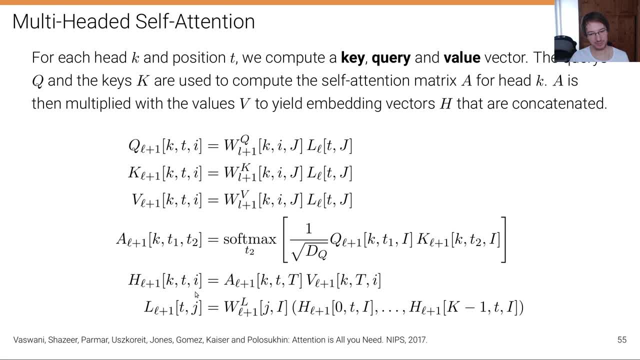 So we get this 64-dimensional matrix And then we compute the dimensional vectors H, which we then concatenate. So this is here over the different hats. So we have hat zero up to hat K minus one. So we concatenate them and then we compute a matrix product. 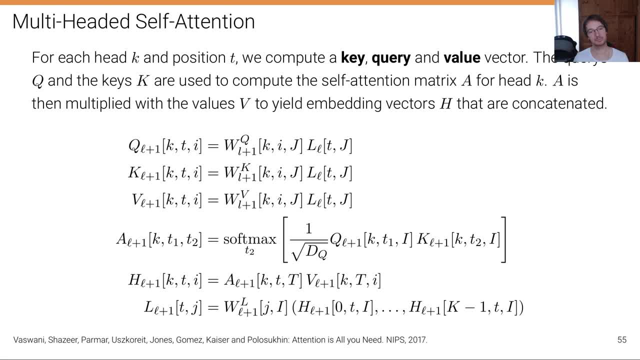 in order to get the output of that layer. And that's it, In summary. we compute queries, we compute keys and we compute vectors. So we take the values for each hat and for each time, step or word, And then, from the queries and keys, we compute attention. 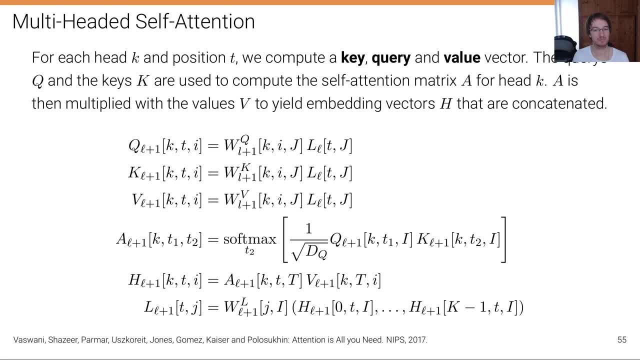 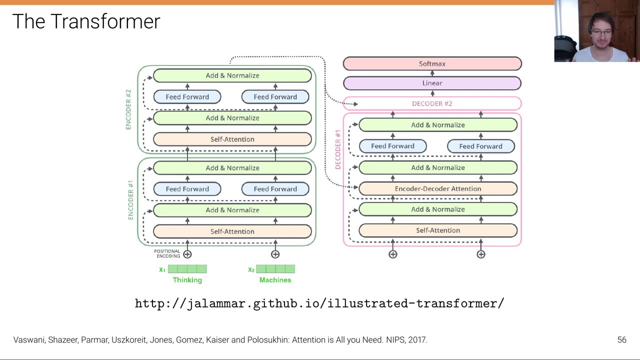 And that attention is multiplied with the values. So we extract, we take the values where the model attends to, And these are then concatenated and fed to the next layer, And here's an illustration of this. This is one that I think is quite intuitive. There's the web link as well. 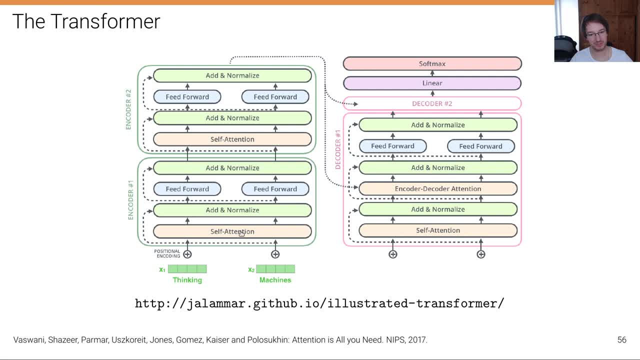 Now, in order to use this, what I've just described is just this self-attention layer. There's additional layers, There's some feedforward layers, There's some normalization layers, But this is really the core of the transformer. And now, if you want to use this for translation, you will have a sequence of input words that are: 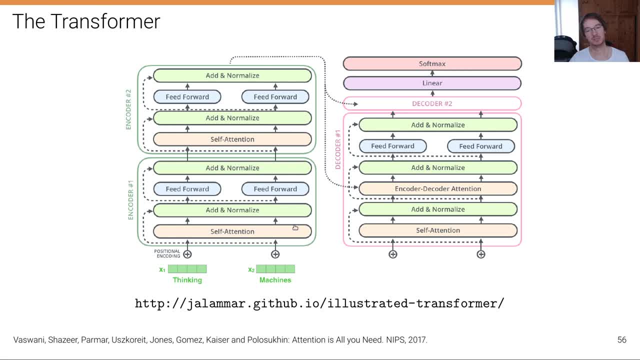 going to be encoded. Here on the left you can see the encoder And then information from this encoder is given to the decoder. In particular, the key and the queries are given to the decoder and they are combined with the values of each word in sequence encoded through this encoder. that's part of the decoder. 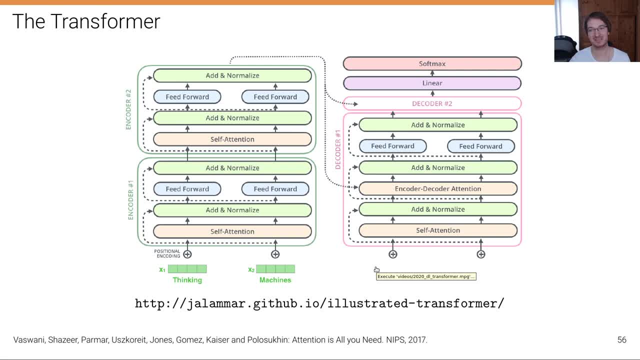 So there's an output sentence here that's successively established through this decoder by combining keys and queries from the encoder with values from this decoder, And this decoder always predicts the next word. And now there's some tricks here, for instance, in order to make sure that this decoder doesn't. 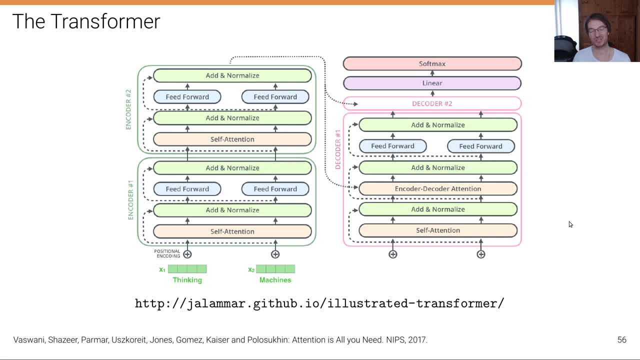 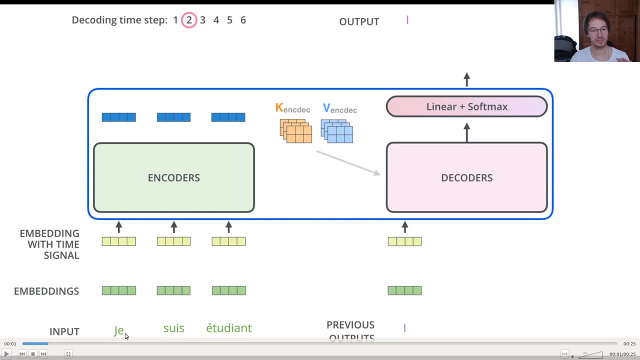 attend to words in the future, because it should only produce one word at a time, like weights in the future are masked out, for instance. So here's a little illustration of how this works. So this is the encoder on the left. It's a translation problem. We have a French input sentence. 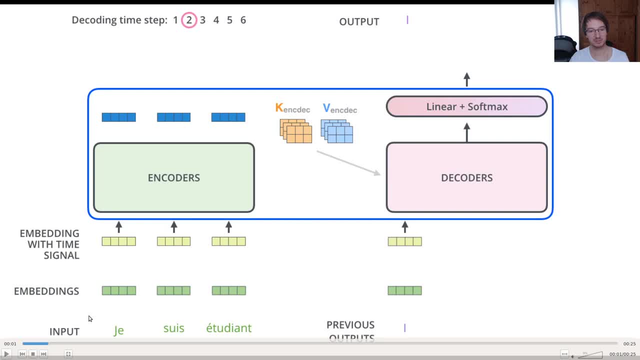 and then an English output sentence, And so the French input sentence is encoded using this stack of six of these transformer layers, And then the features are these keys and the values are basically passed to the decoder and then are queried by the decoder. So actually the keys and the values are passed from the encoder to the decoder, and then the 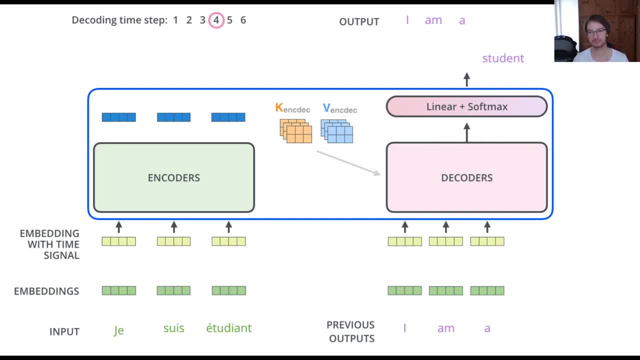 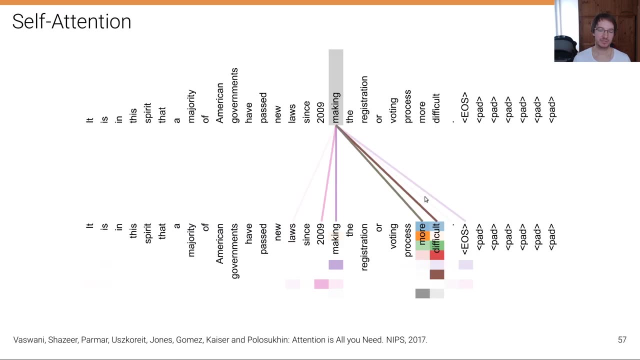 values are combined with the queries of the decoder, not the keys and the queries. So step by step we produce the output sentence, then end of sentence. So here's an illustration of what this attention looks like. So we have a sentence here and we have the word making and we can see for these eight different 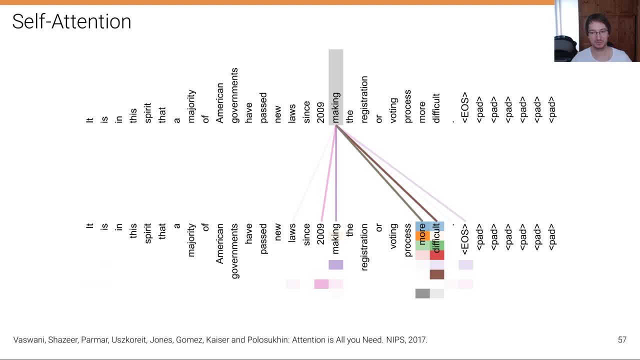 colors. there's a combination of what the attention has shown in rows here. What they attend to is illustrated with stronger colors. You can see that making intense to more difficult more than it tends to our words. So the model has captured that there is a relationship between these two words. 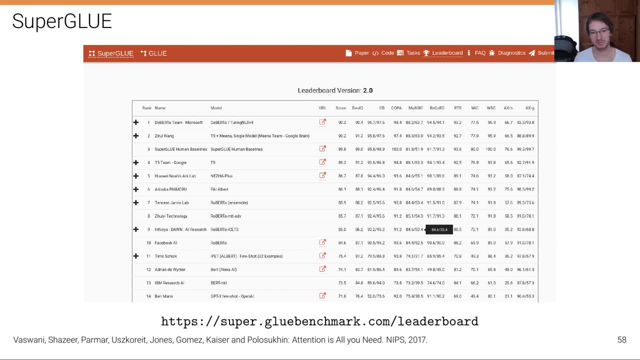 Now, if you look at the state of the art in machine translation, look at, this is the so-called superglue benchmark. you can see a whole bunch of models here that get better and better over time, achieving performance that people thought previously was impossible. and um, all of these state-of-the-art models use transformer architecture. 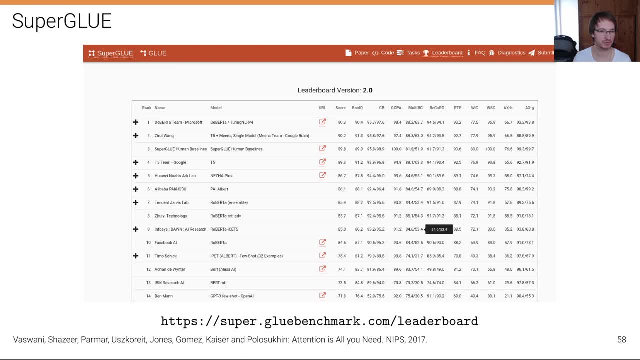 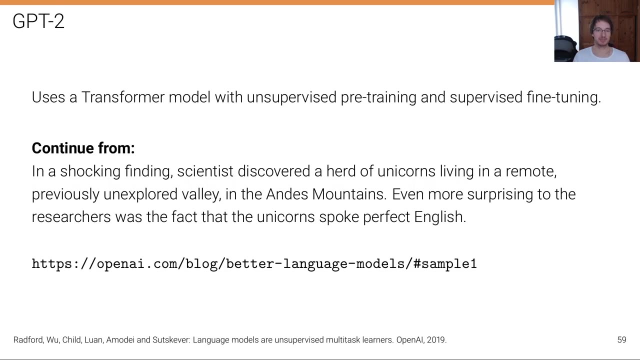 in one or the other way. they all differ in terms of the details and in terms of how training is done and the data sets and the hardware, but they're all building on top of similar ideas. maybe you have heard of gpt2. gpt2 is a model from openai which is basically also just a transform. 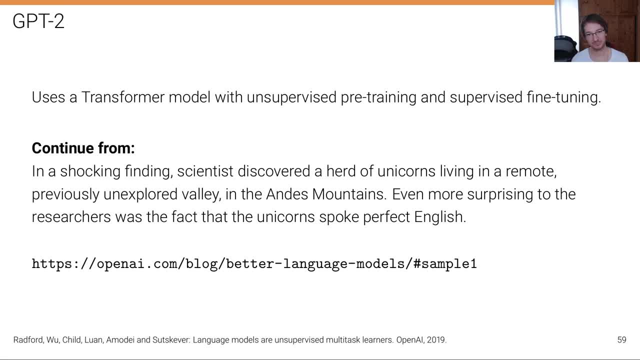 model that they combine with unsupervised pre-training. so we first pre-trained unsupervised on very large text robora with extremely large hardware, and then supervised fine tuning. and they proposed this application of zero-shot learning where the task that is given to the model at inference time after the model has been trained, is to continue from a prompt. so you give 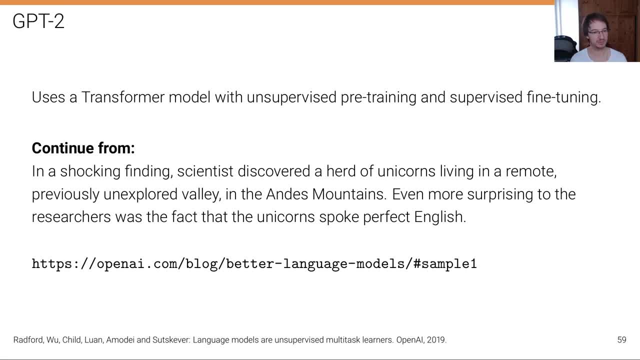 the model, a sequence of words, and ask it to continue from there. and there's a couple of great examples that you can find on the openai website. and this was really- this was really surprising to many- how well this could work. people started to believe that ai is possible, and then they saw this first, 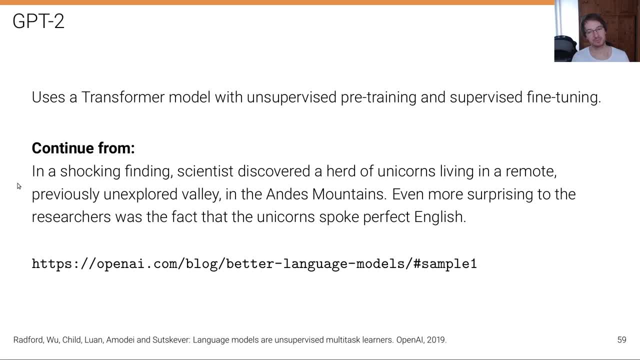 so here's an example. they gave us an input um the following: in a shocking finding, scientists discovered a herd of unicorns living in a remote, previously unexplored valley in the ants mountains. even more surprising to the researchers was the fact that the unicorns spoke perfect english. 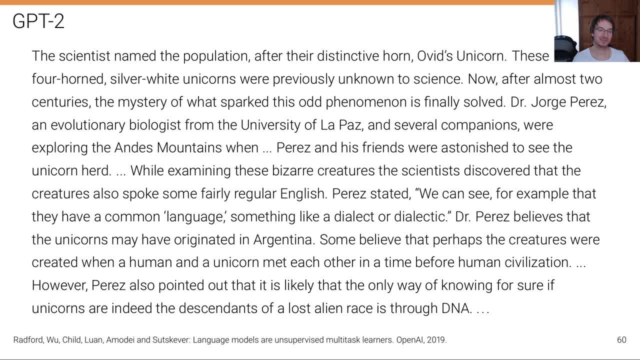 and now this is is the continuation of the machine. This is the machine talking. The scientists named the population after their distinctive horn of its unicorn. These four-horned silver-white unicorns were previously unknown to science. Now, after almost two centuries, the mystery of what? 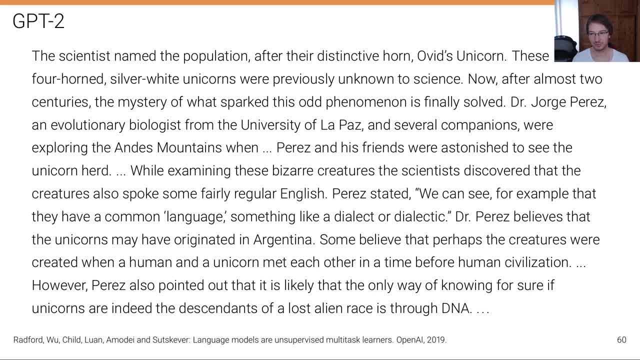 sparked. this odd phenomenon is now finally solved. Dr George Perez, an evolutionary biologist from the University of La Paz, and several companions were exploring the Anse mountain when Perez and his friends were astonished to see the unicorn herd. While examining these bizarre creatures, the scientists discovered that the creatures also spoke some fairly regular 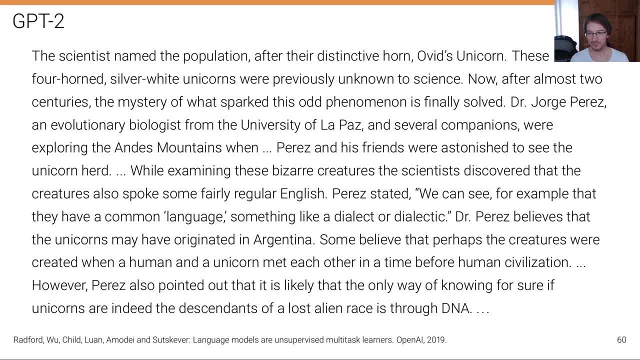 English Perez stated. we can see, for example, that they have a common language, something like a dialect or dialectic. Dr Perez believes that the unicorns may have originated in Argentina. Some believe that perhaps the creatures were created when a human and a unicorn met each other. 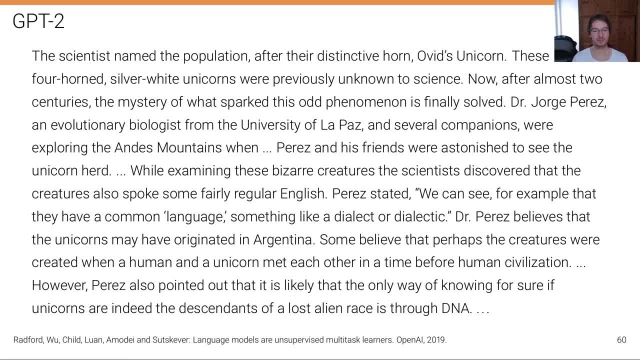 in a time before human civilization. However, Perez also pointed out that it is likely that the only way of knowing for sure if unicorns are indeed the descendants of a lost alien race is through DNA. This was really shocking to many that something like this was possible. 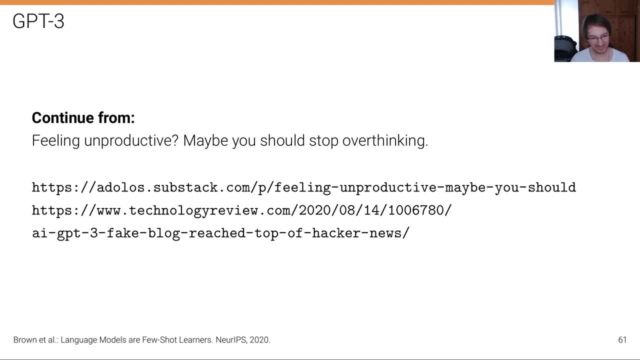 And then GPT-3 is now the new curious incarnation of this system, And there was this famous case of a blogger, an undergrad, that got access to the system and queried the system with very simple queries and then put the results out as a blog post. And that blog post got a lot of press and got a lot. 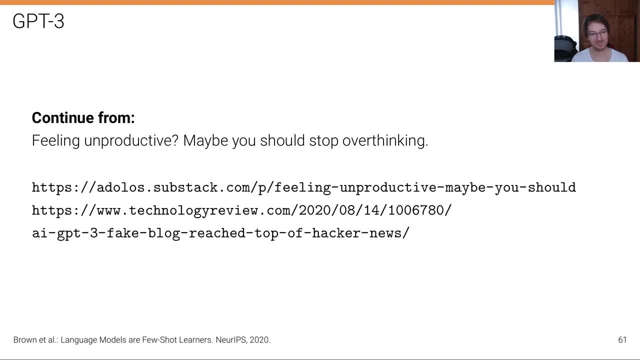 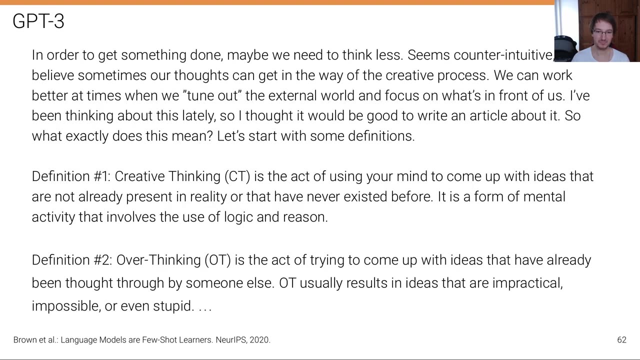 of comments And people didn't realize that that blog post was written entirely by a machine. So here's the input. The prompt is feeling unproductive. maybe you should stop overthinking. And this is what the machine says or produced In order to get something done. maybe we need to. 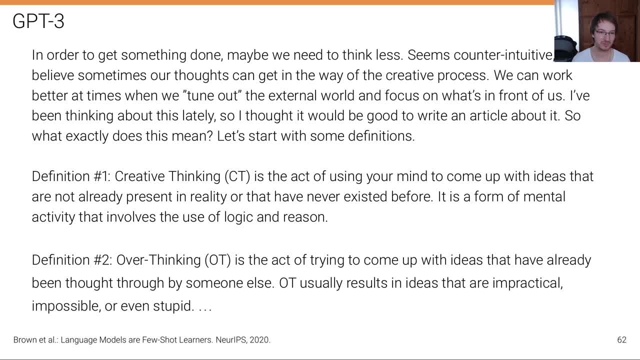 think less Seems counterintuitive, but I believe sometimes our thoughts can get in the way of the creative process. We can work better at times when we tune out the thoughts that we have, Maybe even if we just focus on what's in front of us and not the external world, and focus on what's in front of us. 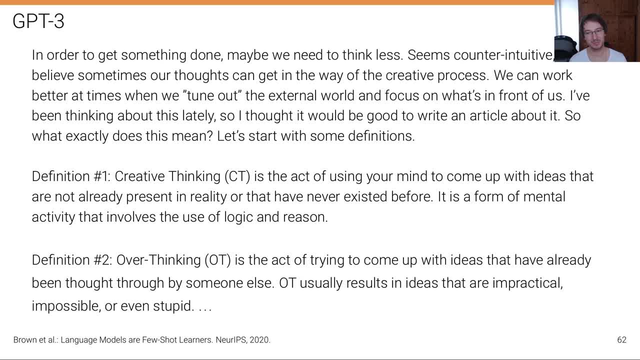 I've been thinking about this lately, so I thought it would be good to write an article about it. So what exactly does this mean? Let's start with some definitions. Definition 1: Creative thinking CT is the act of using your mind to come up with ideas that are not already present in reality or that have never existed before. 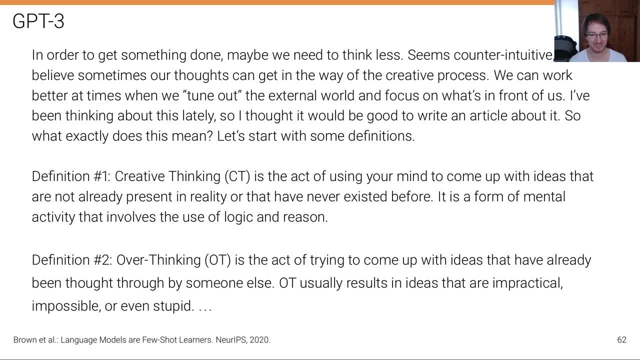 It is a form of mental activity that involves the use of logic and reason. Definition 2: Over-thinking OT is the act of trying to come up with ideas that have already been thought through by someone else. OT usually results in ideas that are impractical, impossible or even stupid, and it goes on. 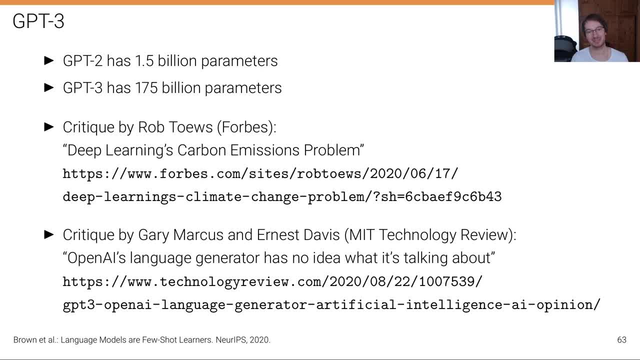 So this was really impressive, but there's also some downsides to these models that I'd like to mention here, And there's several critiques, and I picked out two. So one problem with these models is that this is not the models you might want to train. 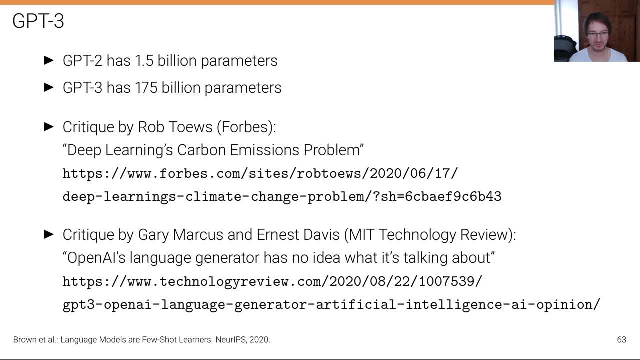 at home. GPT-2 has 1.5 billion perimeters. This was already a huge amount of perimeters at the time. GPT-3 has 175 billion perimeters, more than two orders of magnitude more than the previous model.